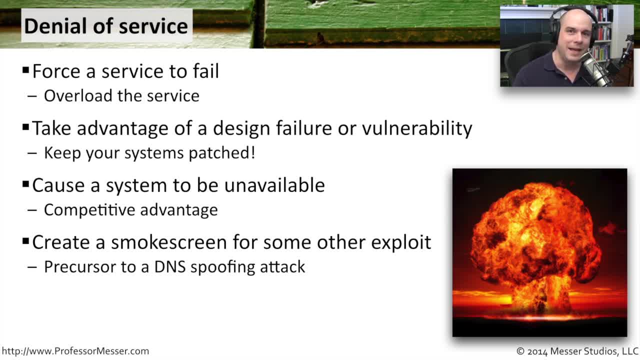 We talked about DNS spoofing, We talked about DNS poisoning, And when you start to do those types of things, it may become very useful for you to create a diversion or to overload a legitimate server, so that you can take advantage of that And you can become the legitimate server. 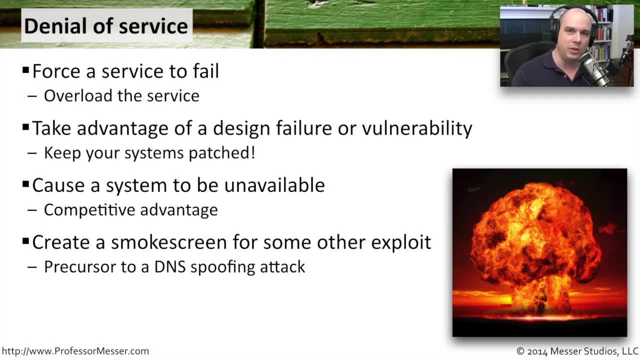 You're now available, That other machine no longer available. You're now the new DNS server And when it comes to DNS poisoning, that can be very, very, very useful, very helpful when you're performing that type of attack. This, of course, does not have to be a complex process. 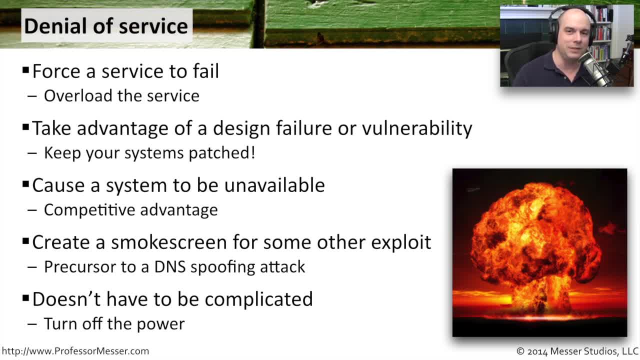 for denial of service. I mentioned the very basic definition of a denial of service is to prevent any access to that resource. One good way to do it would be to turn off the power. You don't have to have a million systems hitting a web server. 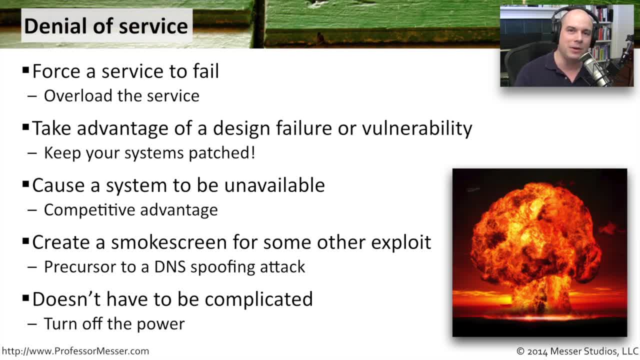 at once. You simply go outside the building. You notice outside of the building the power, the big switch for the power system on the building is not locked up. You walk up, You turn the switch, The entire building goes down. You've just created a denial of service situation. 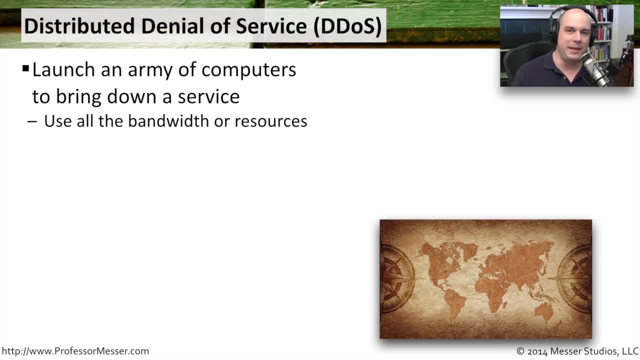 When we're talking about big time denial of service, though, we're talking about many devices on the internet participating all at once. Whenever we were looking at botnets in our botnet video, we were talking about these botnets just sitting there and waiting for a command. 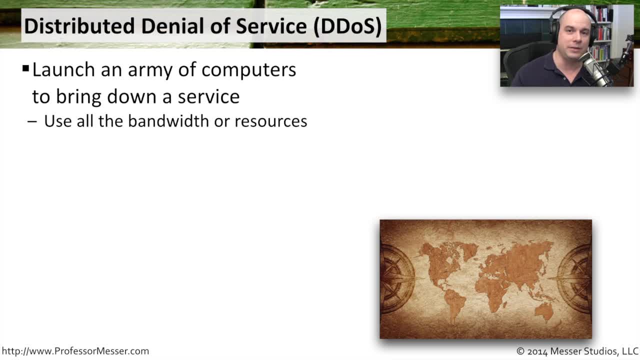 And the bad guys may take an army of their robot network devices out there. send them a command that says: please take down a web server. Send a denial of service attack to a particular site, And so you can use this army of computers to bring down that service. 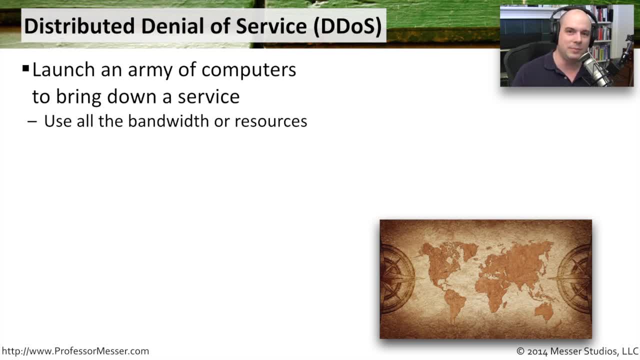 Use all of the bandwidth, Use as many resources available in that web server. If that web server can serve 1,000 users at once, hit them with 2,000.. He'll be so busy trying to serve that many systems he won't be able to operate and do anything for anyone else. 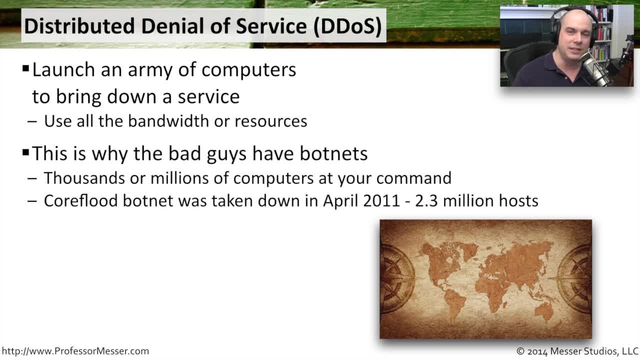 This is exactly the purpose of a botnet: not just to send spam, but to participate in these massive types of events. CoreFlood was a really good example of this. This was taken down in April of 2011.. 2.3 million devices, it's estimated. 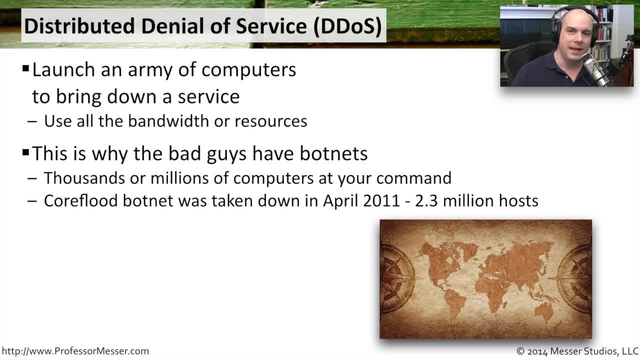 were participating in this CoreFlood botnet And these botnet command and control would send these devices out. to take down individual systems Becomes a bit of an issue when you're trying to keep those websites up and running. There's really very little you can. 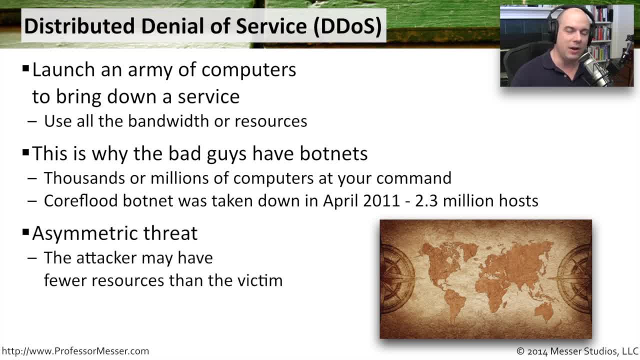 do when that many systems are hitting you all at once. This may also be something called an asymmetric threat, which means the attacker, the individual device, has fewer resources than the victim has. Sort of an odd situation. You've got all these individual boxes out there. 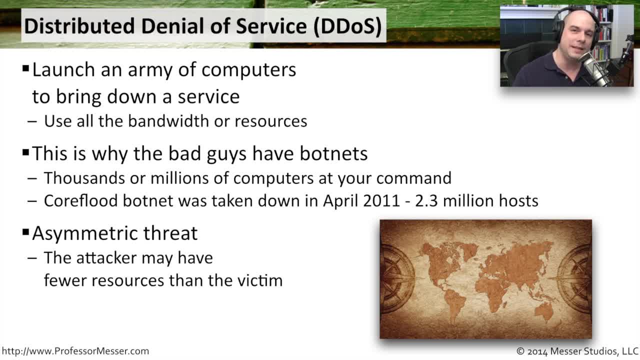 They may be very tiny devices, but they're now all working together to take down a much larger giant. That becomes a real big issue. It's very difficult to build a web server that would be able to accommodate 2.3 million requests all at once. 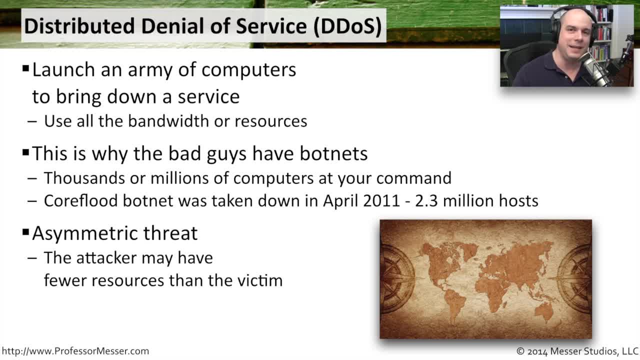 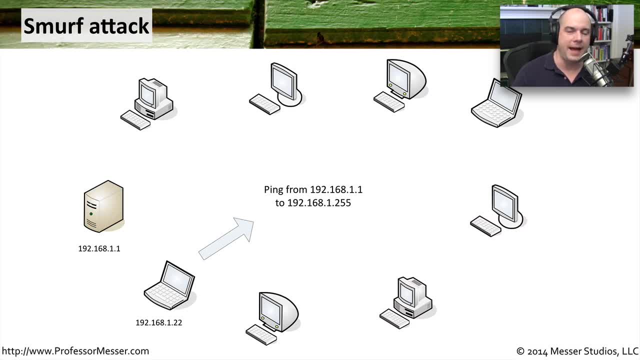 And therefore it's very, very simple for these tiny, tiny little devices to take down those monster websites. One of the very first in all of service attacks was one called a Smurf attack, And what was nice about the Smurf attack is you could get a lot of bang for your buck. 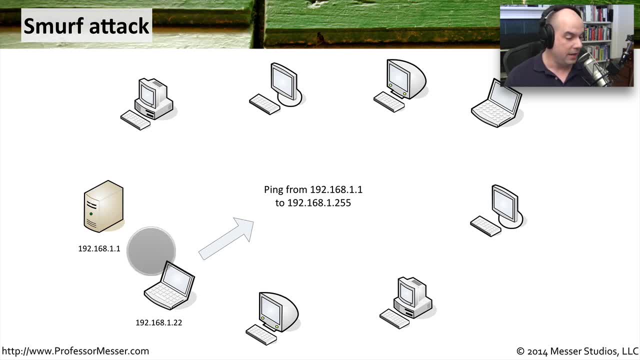 And here's what I mean by this. You would be a station out on the network- 192.168.1.22, let's call you on this laptop- And you would like to take down this server that's at 192.168.1.1. 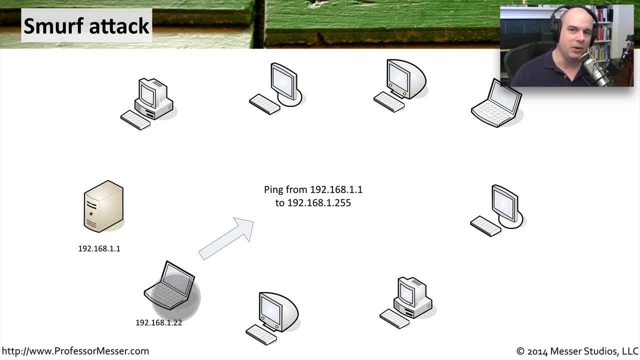 But one machine that's sitting out here would be very, very difficult, because this is a big beefy server. it would be very difficult for one machine to take down that one server. So the key to a Smurf attack is that you. 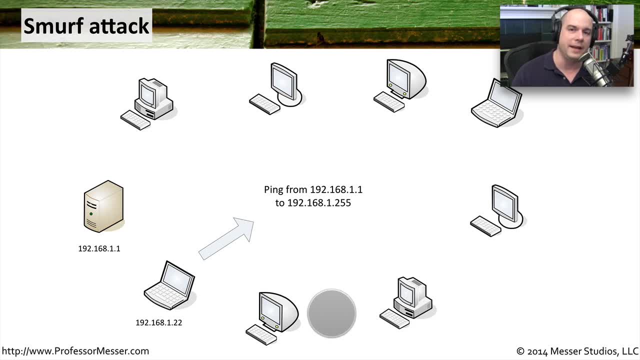 get to involve everybody else on the network, And the way you do that is through something that was very commonly done back in the day. This was back. This was back in the 90s. This is a capability that really, you don't see much anymore. 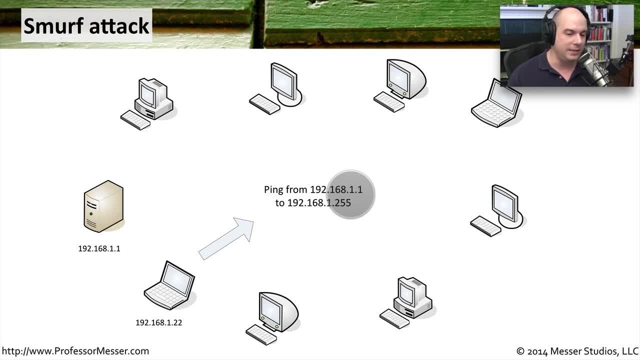 But you send a ping out, an ICMP echo request. Then you spoof the from address, Even though you're 1.22, you send the packet out and say, hi, I'm 192.168.1.1.. You pretend you're the server. 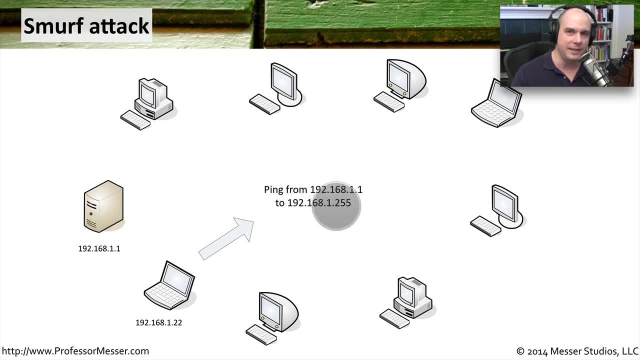 And you send it to the broadcast address for the subnet. When all of these devices out here see this packet, they are all programmed to take and react to broadcast addresses. Everybody must look at a broadcast frame. That's the whole purpose of a broadcast.